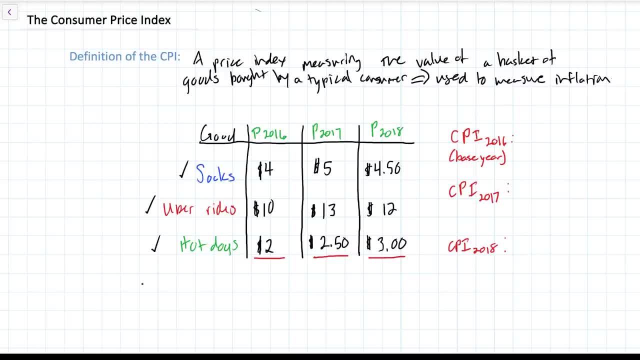 oversimplification. In a real country, consumers would buy all sorts of goods. For the simplified example, however, we're assuming that the typical consumer only buys these three goods. What we have here are the prices of each of these goods over three years, in 2016,, 2017, and 2018.. What 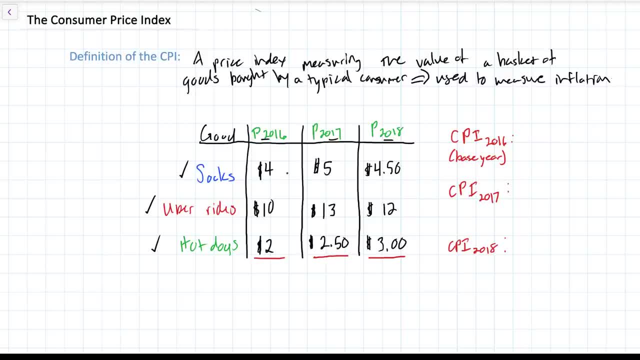 we're going to do is add up the prices in each of these years to come up with our price index. We're going to add up the prices in each of these years to come up with our price index For the basket of goods over three years, and then we're going to calculate the CPIs for each of the 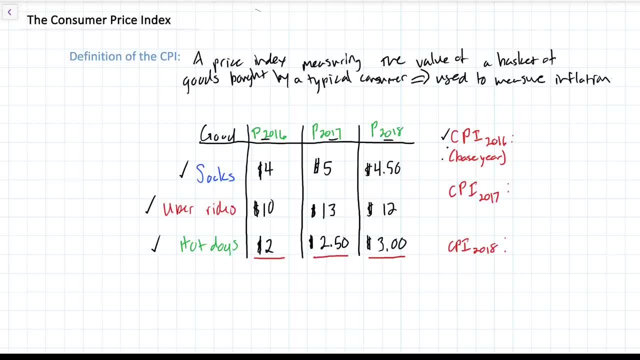 years, using 2016 as our base year. First, let's add up the total values of the basket of goods consumed by the typical consumer in each of the three years. What we can do now is calculate the CPIs, or the consumer price indexes, for each of these years. The formula for the CPI is the price. 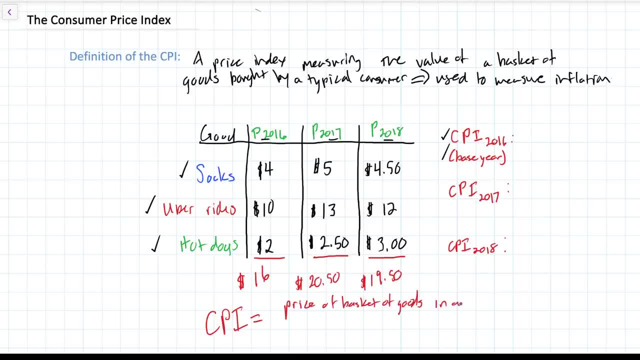 of the basket Of goods in one year divided by the price of the same basket of goods in a base year. Since we are talking in terms of indexes, we must multiply this by 100 to get our consumer price index. We can actually go ahead and calculate the CPI's for each of these years. now We know that the base 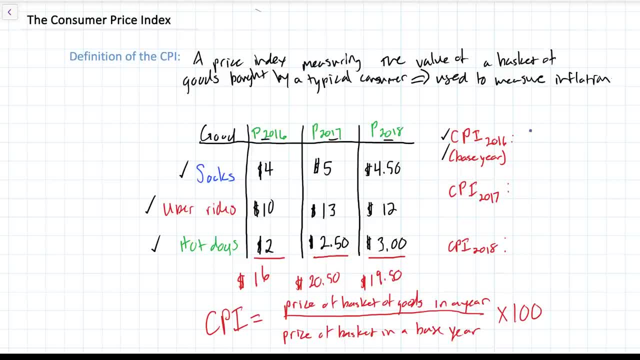 year is 2016.. So the CPI for the base year is super easy to calculate. It's 16 divided by the price of the same basket of goods in one year, divided by the price of the same basket of goods in the next year. 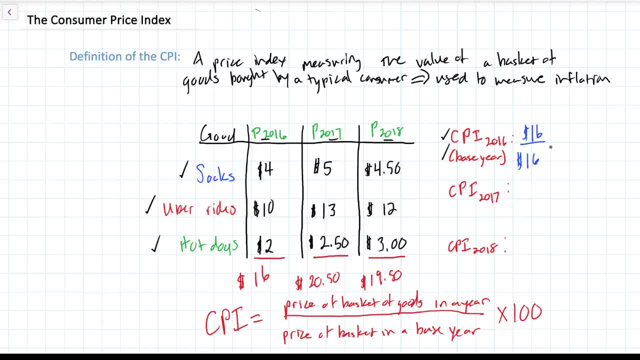 in 2016,, which is $16, times 100.. So we get 16 divided by 16 is 1 times 100.. The CPI for the base year is clearly 100.. This is the basis on which we can calculate changes in the CPI and determine how much inflation there is in years moving forward. For 2017,, we had a price of $20.50.. We can calculate the CPI by dividing the price of the basket of goods in 2017 by the price of the basket of goods in our base year of $16 and multiplying that result by 100. Let's do that. 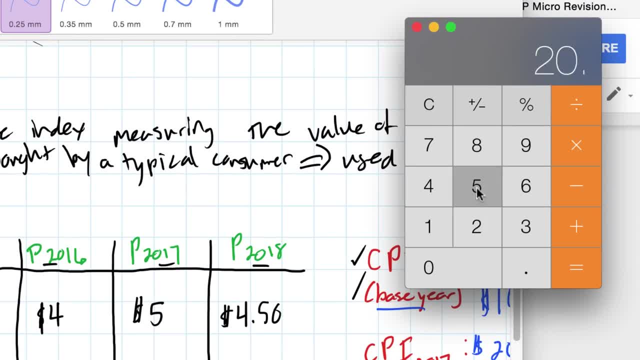 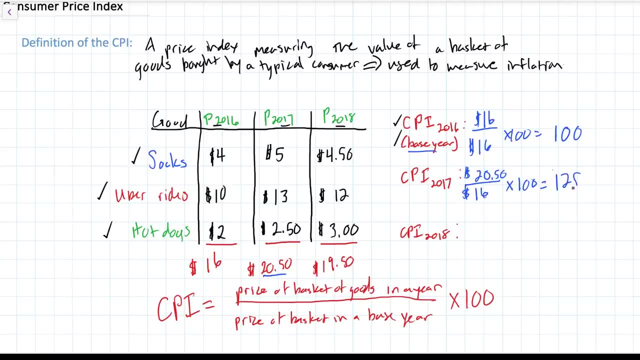 calculation now. Okay, we've got: $20.50 divided by $16 gives us 1.28.. Multiply that by 100 and we get 128.125.. So the CPI for 2017 is 128.125.. We're just going to round that to 128. for the sake of sense, Now we can calculate the CPI for 2018.. We take the price of the basket of goods in 2018, that's $19.50, $19.50, and divide it by the price in 2016,, which was $16.. We'll multiply that by 100.